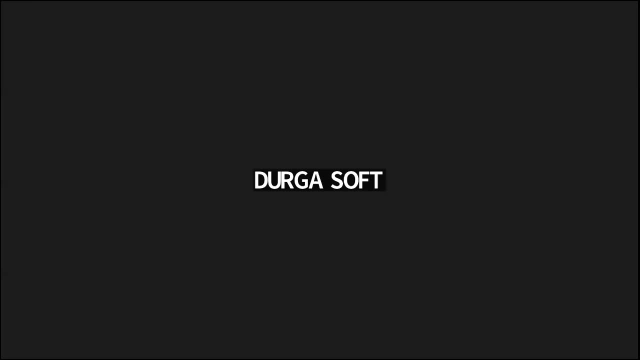 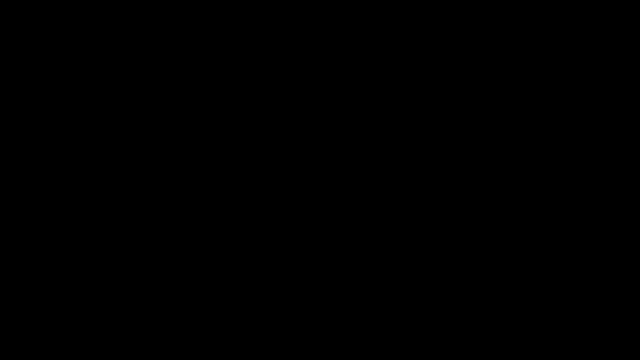 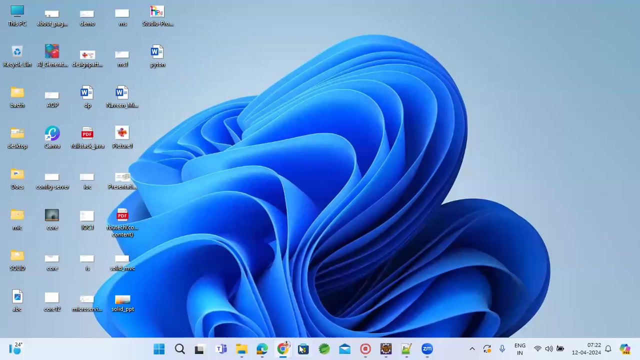 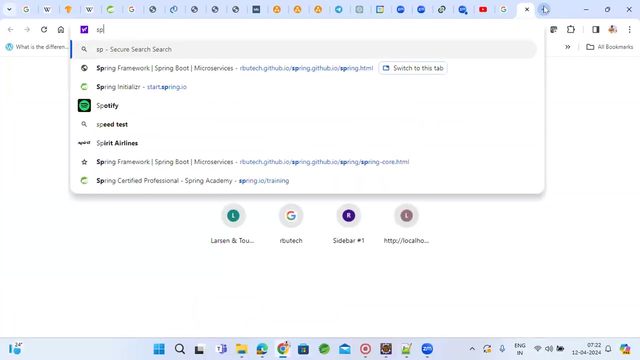 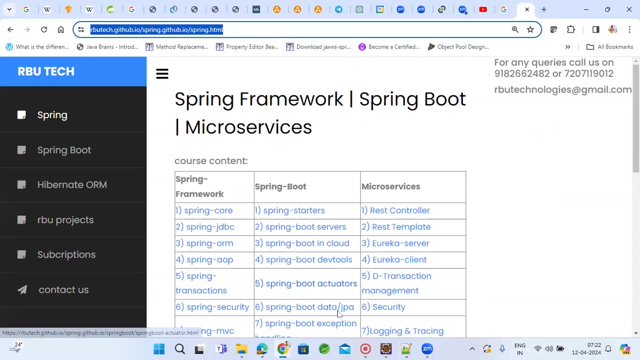 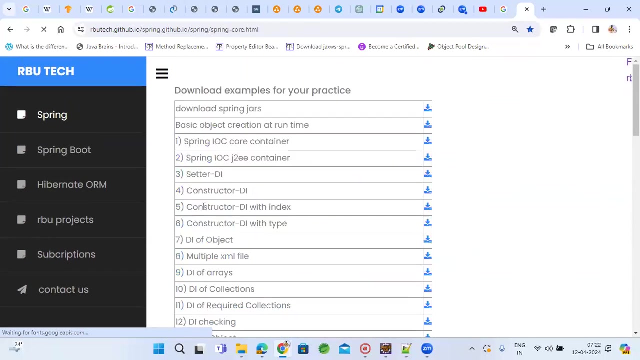 Okay, yeah, I can able to share my screen. Hope my screen is visible. Yeah, So here you guys. please go through this link. Okay, We have course content here. Okay, I shared you one link, Course content you have here and course examples also I have given here, just for a reference. 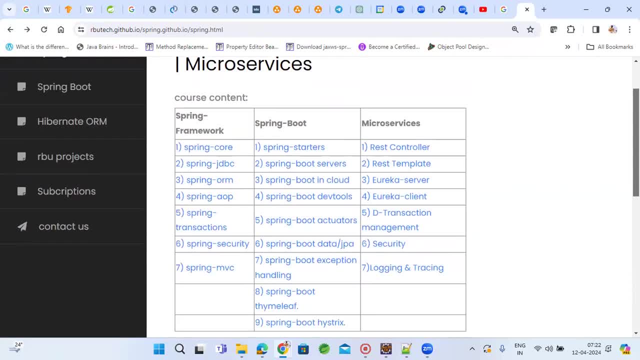 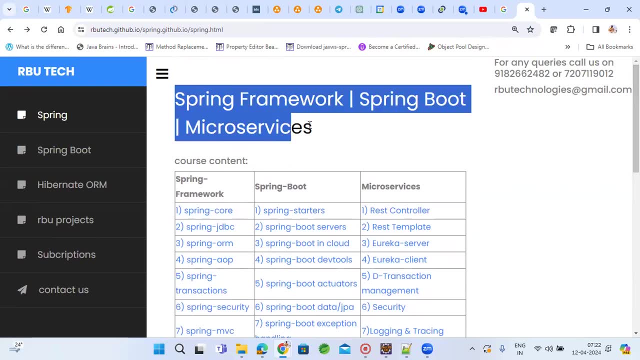 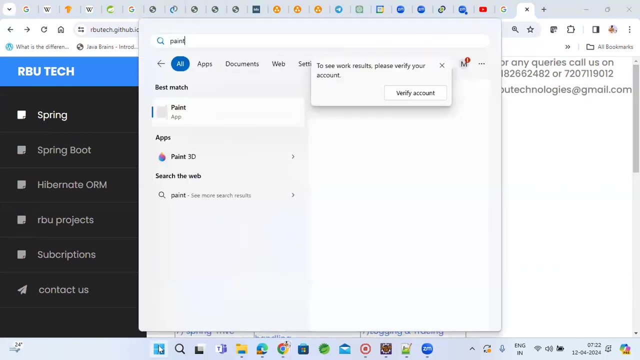 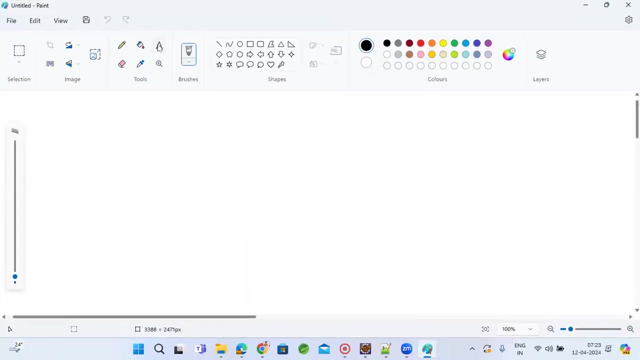 Okay, Yeah, Coming to this program. right, We are going to share you both: Spring Framework, Spring Boot and Microservices. I'll be covering As part of this training. I'll be covering all these three concepts: Spring, Spring Boot. 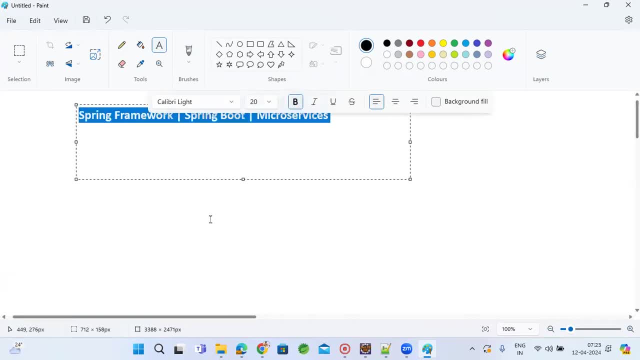 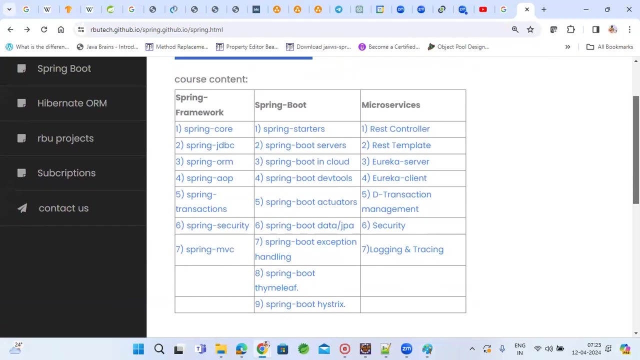 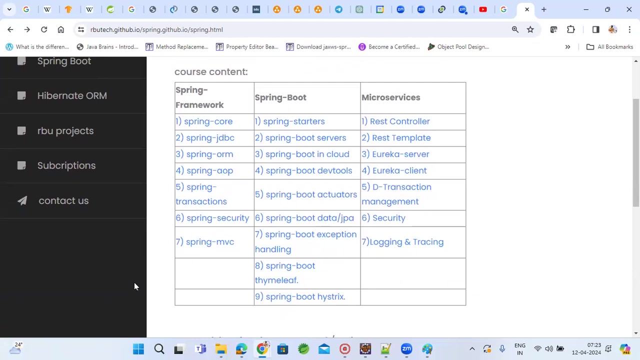 and Microservices. Okay, So Spring Boot is advanced version of Spring Framework and using Spring Boot, We will be covering Microservices concepts and Microservices design patterns, everything Okay. Coming to the topics, you can see this list here. You can see this list. Okay, Just a minute. 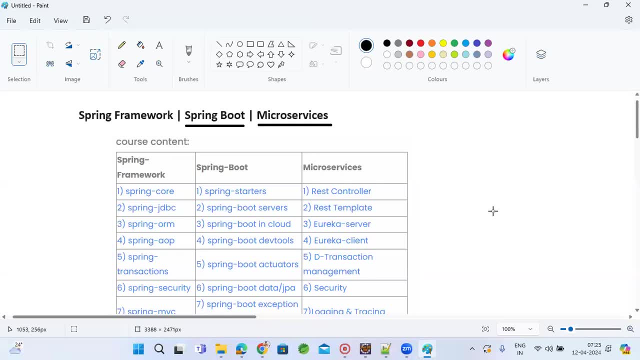 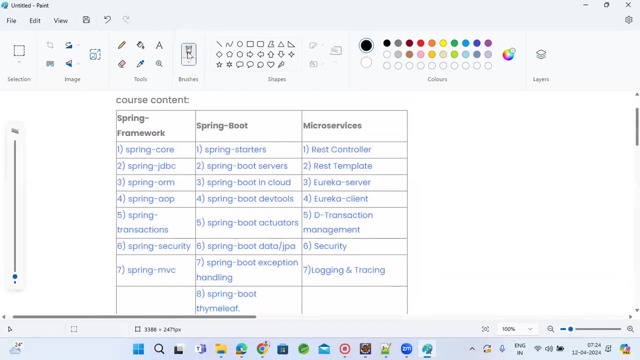 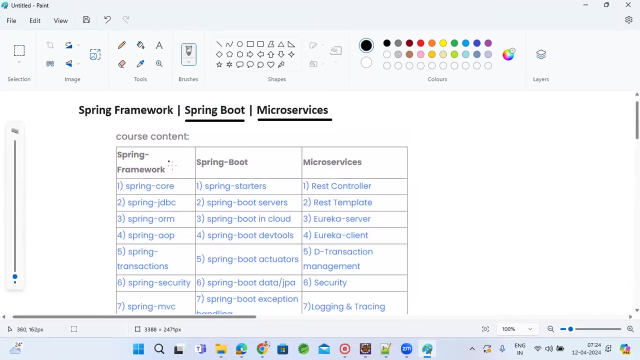 Yeah, We will be starting with Spring Framework. So if you not aware of Spring also no issues. From the beginning, we are starting. We start with the Spring Framework, Starting with the Spring Core module, Starting with Spring Core module. So here you will learn all the basics of Spring. 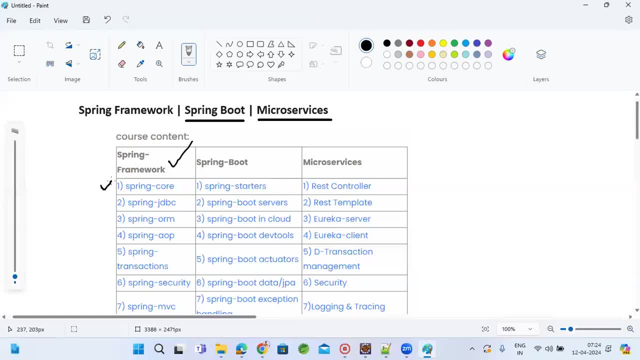 as a framework, how it is build, how it works, how to do configurations, annotations, dependency, injections- lot of concepts. we have part of core, so you will get strong foundation here, first with core module and on top of it, spring JDBC module and advanced spring ORM, spring AOP. how? 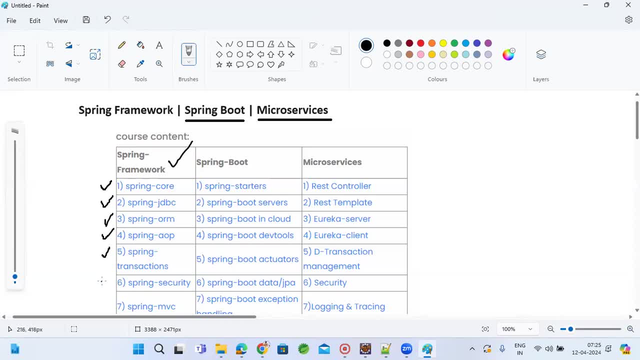 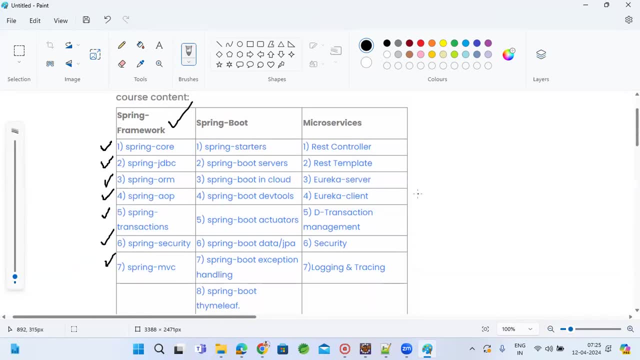 to handle transactions in spring. security and MVC will be covered here. okay, so once we done with the spring framework we jump into spring boot. I'll be covering all the spring boot concepts, from basic to advanced level and micro services. so this journey, totally you know we will take around. 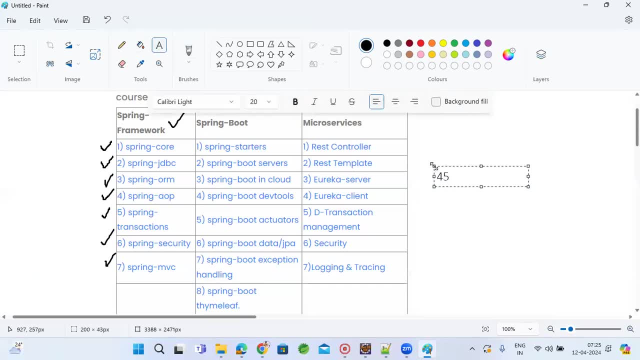 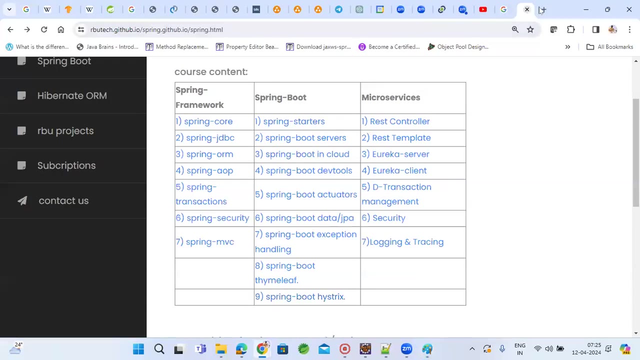 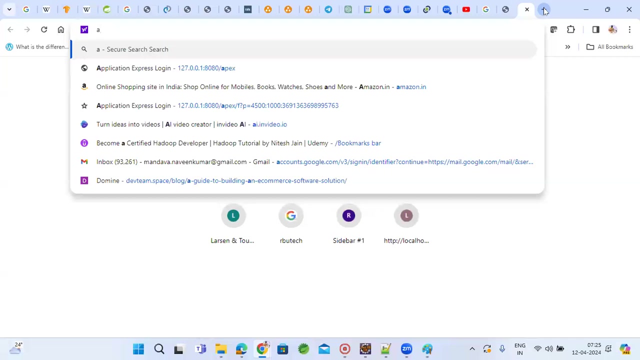 45 sessions, 45 plus sessions required, okay, and it may go around two months course, okay you. so this thing Y lies makes data looping borrow from technical data breatheiv pro donné is not that? if you have seen three software demo videos also that are available, I'll share a link if you want to quickly go through it. 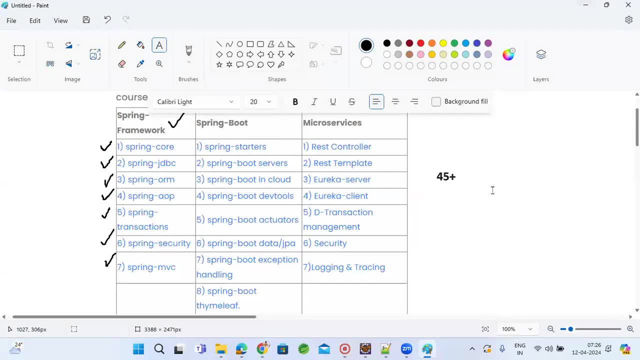 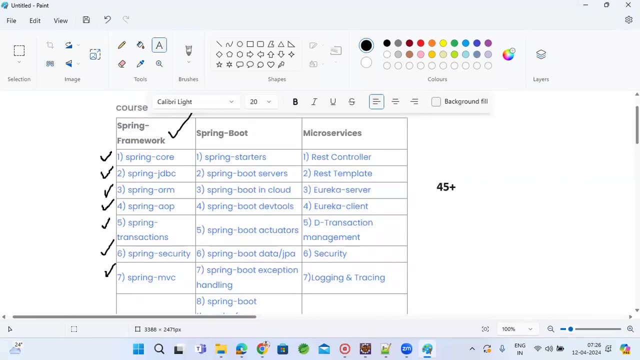 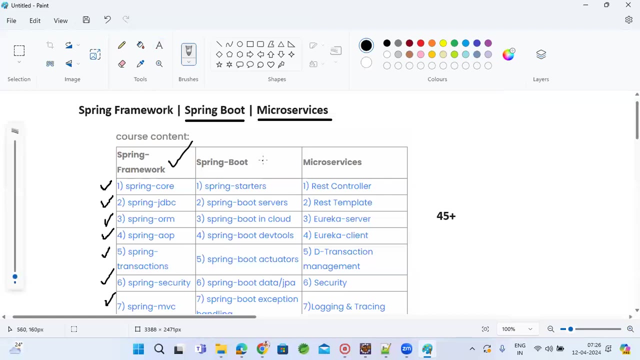 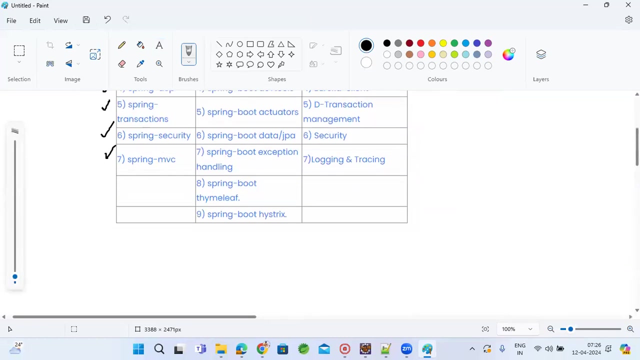 okay, end of the session. I'll share. you can go through the list of demos from that link. okay, yeah, so this is the content, right, very clear. we are going to cover spring, spring boot and micro services, all three concepts. okay, starting with the spring and the basic prerequisites. here is, at least, if you 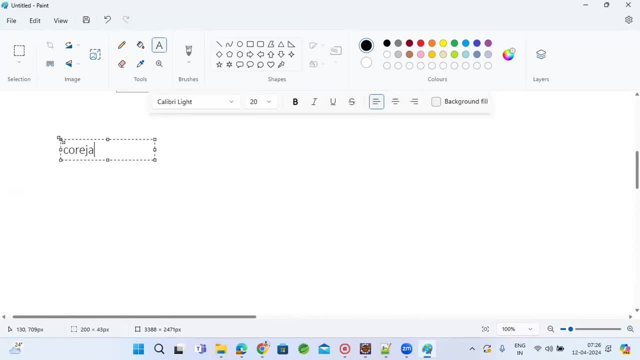 have core knowledge prerequisites, right. if you have core Java knowledge, that is more than sufficient. and if you have advanced Java satellites knowledge also, that is well and good. okay, core Java knowledge is mandatory, so the skill is required and this is optional. but if you know, that is well. 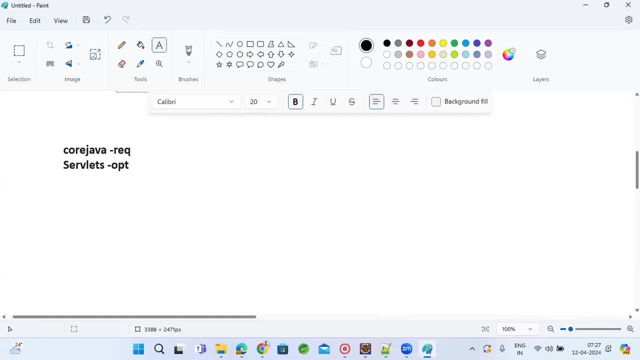 and good, okay. so yeah, on top of it, on top of core Java, we can start learning spring framework, starting with MVC. okay, I'll starts with MVC- right, how to build classes using MVC- and we'll describe about simple for so classes, simple bean classes, right, and how to create objects in simple core Java: object in Java, how to deal with it. 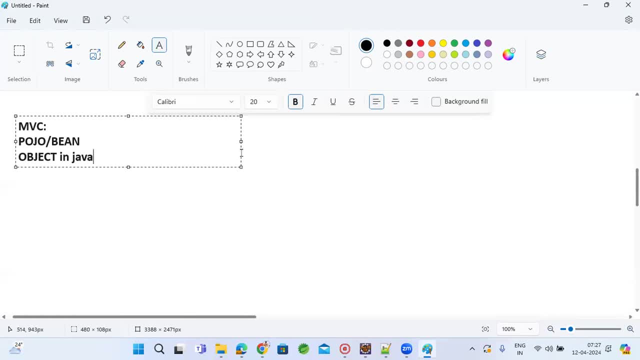 how to create objects, how to connect with them. then we will start with spring core module. as part of core module, we will be going to see containers, we'll see ioc containers, how they will take responsibility of objects. in spring we'll talk about ioc containers here. then there itself we will cover, you know, two design patterns. 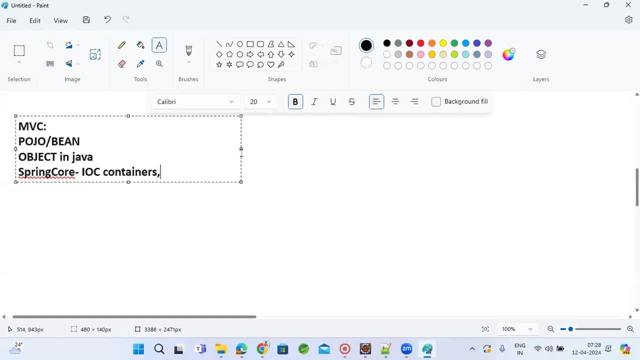 what is singleton and what is prototype and dependency, injection, auto wiring, and we'll be going to see xml based. all these concepts. okay, xml and annotations, xml and annotations. okay. so we'll be seeing two approaches for this, for every example and a lot of stereotypes. we have annotations. okay that, all annotations. 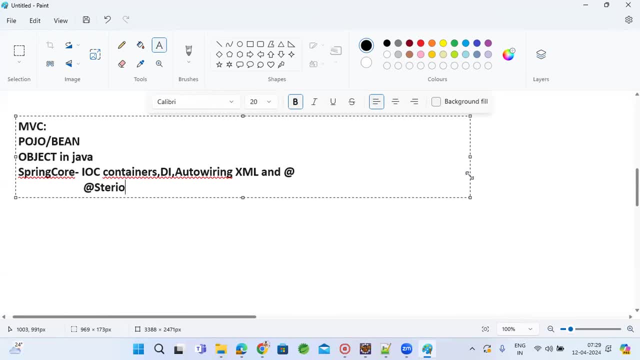 are going to covered here all stereotypes which are very important: how to deal with the properties. okay, how to deal with properties, properties, files. that all we will be learning here. and then we will jump into jdb, jdbc module, which is advanced spring jdbc, which is advanced module for what it is advanced. 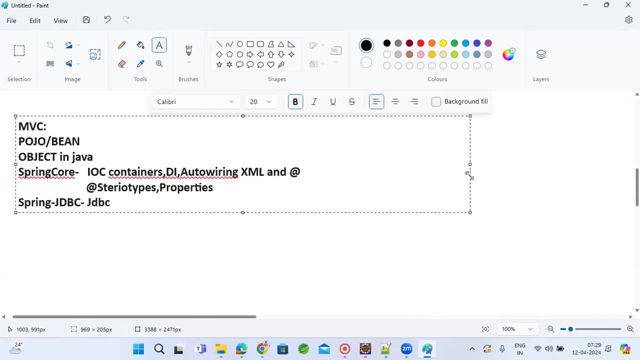 if you aware of jdbc right plain jdbc. on top of that plain jdbc, spring jdbc, given okay uh for production based applications. simple jdbc code is not sufficient and there are, you know, issues that uh you may see in the applications right uh, like connection leakages or insufficient connections. 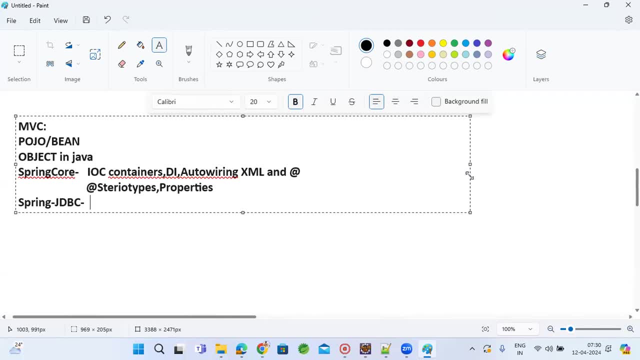 a lot of such issues and performance issues you may see in spring jdbc. we will learn here to avoid all that right connection pooling concepts. connection pool- a lot of connection pools will be covered here, like uh, apache, dbcp and driver manager data so, or a tree manager or落чун from a lot of devices is covered here. okay, so let us talk. 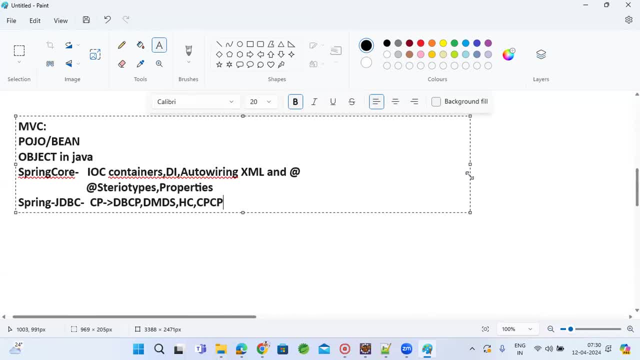 about that, even though these are not all the things that we are going to be using this time, that we are going to be using jdbc, for jdbc and for jdbc. what we are going to be doing is, uh, we will see how to use jdbc. we are going to look at this also- the applications. 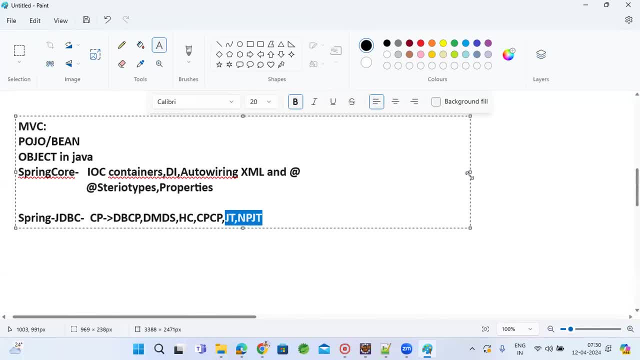 and features too right. so we are going to be using jdbc and actually a lot of them are template classes, so that we are going to see using connection, pool and template classes. JDBC becomes simple to us so that we see here in the spring JDBC module and the next module is spring warm, spring warm, okay, so prerequisite: 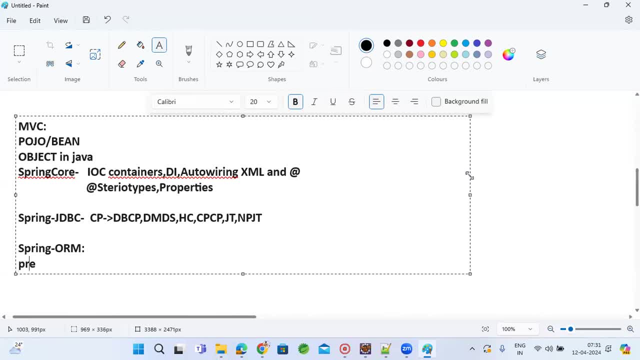 for this. ORM is prerequisite for ORM module is you need to know hibernate. you should aware of hibernate, okay, so I will take one session for hibernate here. I will be covering it. okay, one or two sessions I'll be conducting here. so if you're aware, it is well and good. if not, nothing to worry, I'll be. 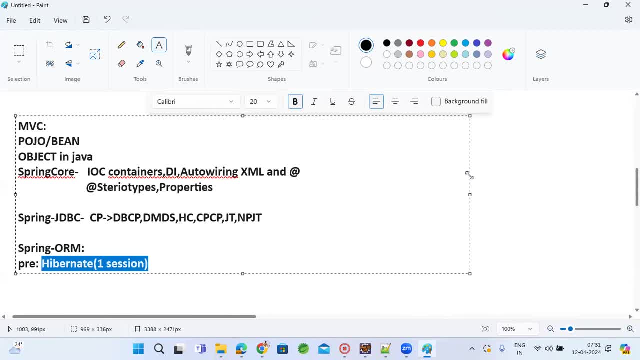 taking hibernate session also as a framework. Hibernate Session is here. you have access to program studies in какanu. you need those net. how it is build. what is the use of hibernate. how to create mapping files in hibernate to do credit operations right. how to do basic crowd operations on hibernate. 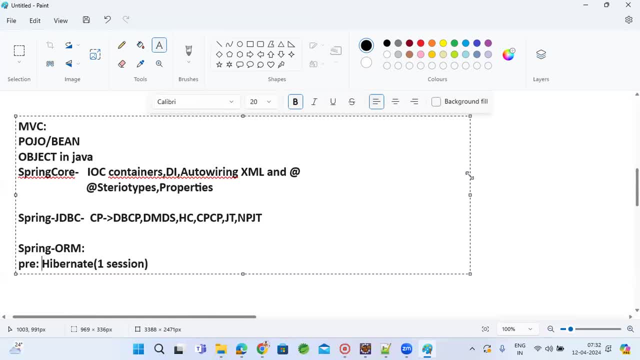 that i'll be covering. if you know, that is well and good. if not aware, also it's okay. i'll give how it will function. okay, i'll take a session for hibernate. then on top of it, in spring warm, right on top of it, we are going to see how to use the xml based. 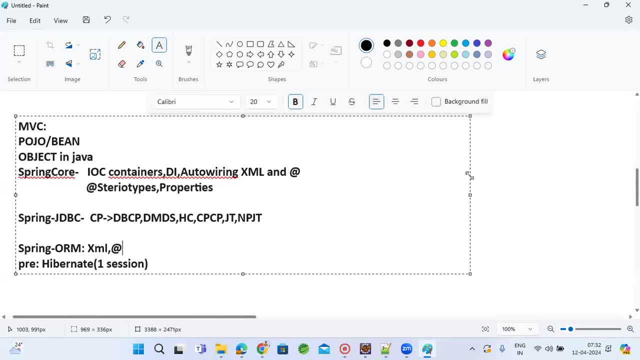 mappings, how to use annotation based mappings here. particularly in warm we do mappings from, you know, java to database. so all that database mappings we will be covering here. and yeah, there are some factory classes, also annotation based factory and xml based factory, some factory design patterns they have used here. so 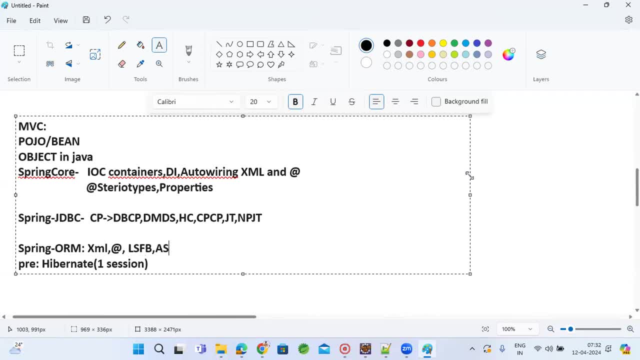 local session: factory bean- annotation session: factory bean: basically why this factory bin classes is: session is important, session is important in hibernate, session is like a connection okay. so to get that connection we use this session factory bin classes. why we need these factory bin classes means spring framework need to integrate it with. 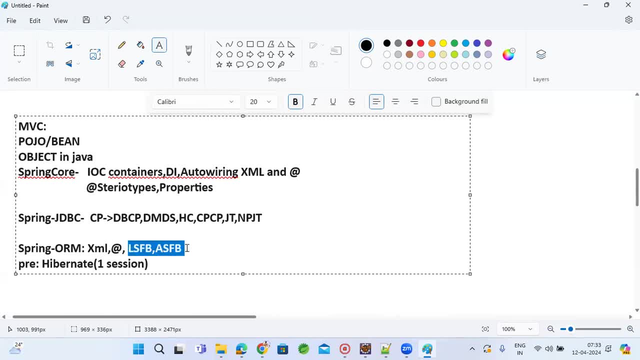 the hibernate frame work. okay, so this classes we use to integrate these classes. we used to integrate two frameworks. okay, so that integration. you will be learning here how to integrate a framework with another framework. basically, that's not a big deal. okay, so using this factory bin classes, we do that. 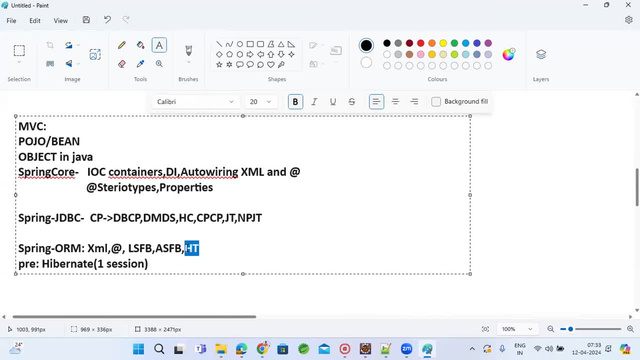 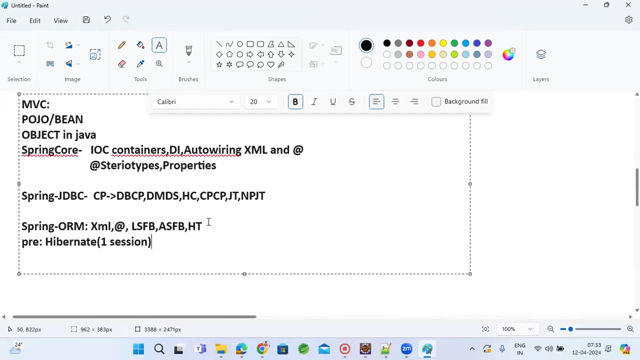 and advanced do using hibernate template. we do make you know making hibernate operations are hibernate itself is simple, but they made it right easy in hibernate template. so that is also we are going to see. and what next? just a minute. the next module: spring aop aspects oriented programming. 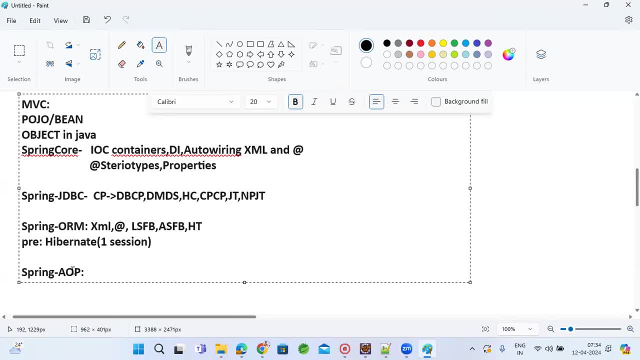 okay. so here we will achieve in this aspect oriented programming right more reusable. or you can say on the fly, we can add aspects services. we can add to business services. we can add to business business like logging, mailing, SMS. if you have any add-on services, that if you. 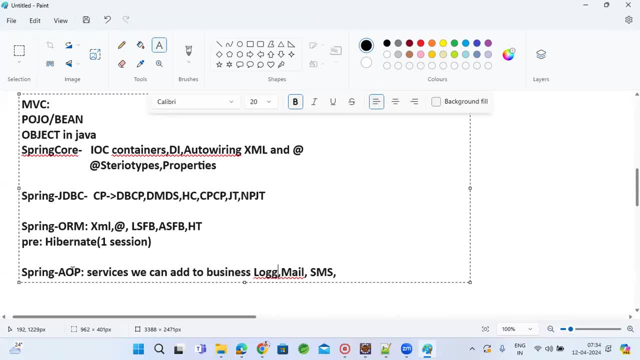 want to add to your business on the fly without interrupting your business, you can. you can add the code so generally, without AOP it is not possible, okay, without interrupting business or without writing logging code. inside business achieving logging is impossible, but in AOP we can. we can do that more reusable. 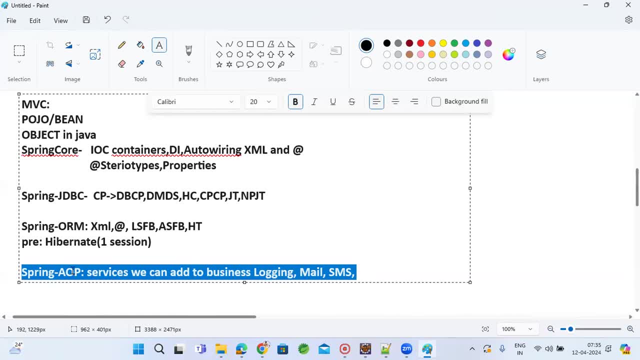 right, it is more reusable. I can write one log component that I can apply everywhere, okay, on the fly, like a filter. I can apply using AOP in one place. I can put the logic that will apply it to all the classes or my required classes easily. okay, without interrupting or without disturbing existing logic. 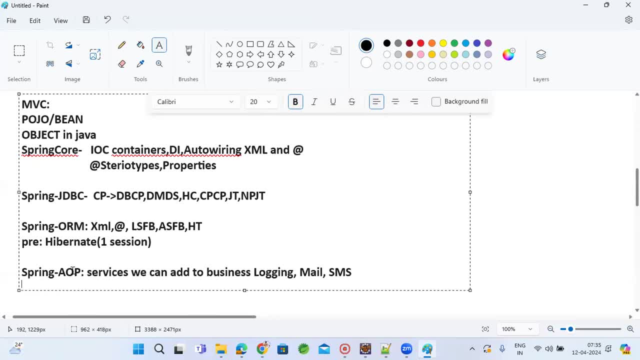 so here we will be covering aspects, how to create aspects, how to add to business logic. so mostly we will see here proxy design pattern- okay, how that proxy will work and aspect oriented programming we learn here. okay, it is more you know useful. who knows AOP will write code in a. 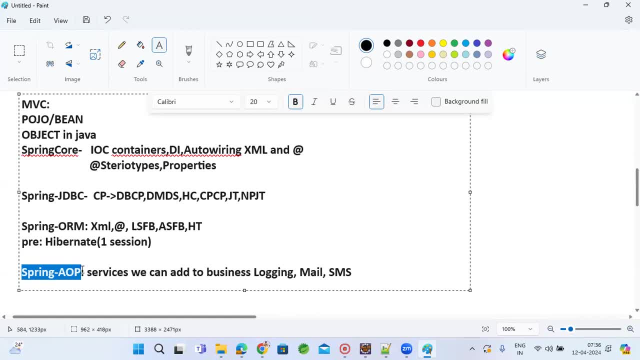 different way. reusable components and all. okay so and easy to use understand also. so four modules covered right and next spring transactions: how to handle transactions in spring when there are, you know, multiple crud operations. right, if you are in a single transaction, in a single transaction, if you are dealing with multiple crud operations. 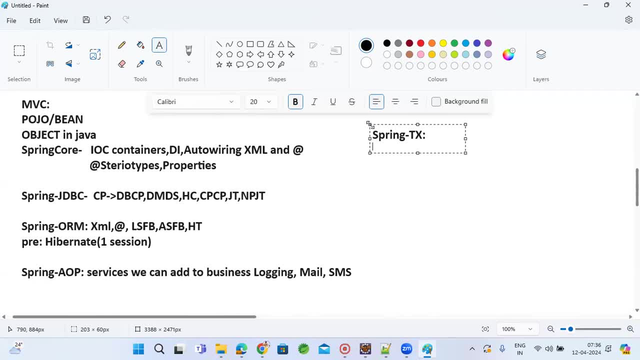 in other words, if you are doing multiple inserts or multiple updates into many tables, if you want to maintain consistency in your data, transactions are really mandatory, okay. so how to handle the transactions? how to handle the transactions, we will be learning in spring transaction module and spring security. we will learn this after spring mvc module, spring mvc designed for. 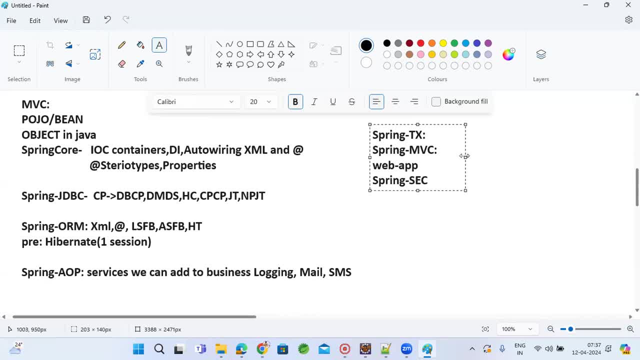 web applications. so if you want to build a web app, okay, how to build that web app using Spring MVC. here we learn right how to configure dispatcher servlet. how to configure dispatcher servlet and how to do mapping- front end view to back-end controller mappings- that all we will be learning here. 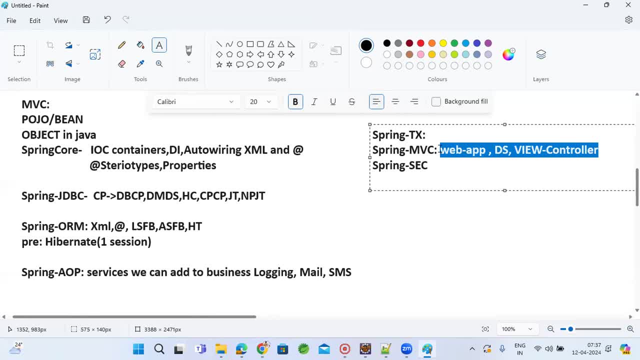 in mvc, so complete end-to-end web application. you can design, post mvc and to apply authentication and authorization. okay, security, to apply security. we will learn spring security module so that you can understand how to you know, authenticate a user and how to give permissions- permissions like authorization. 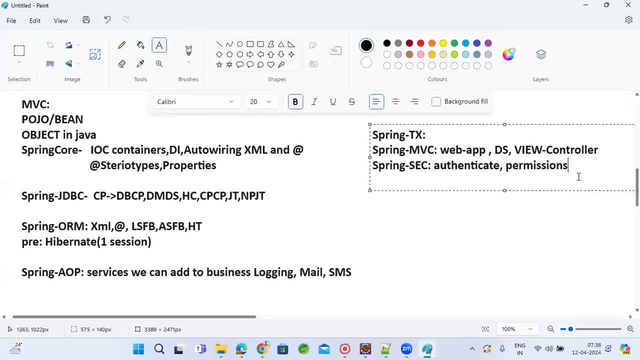 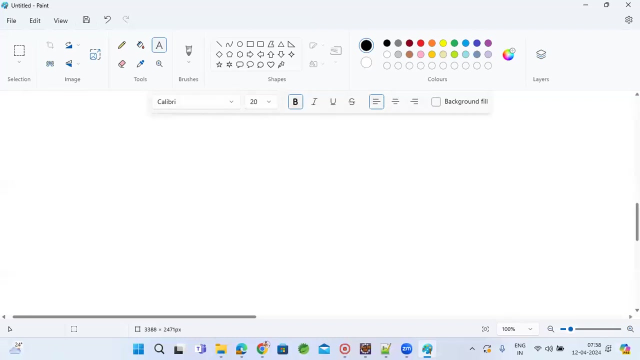 authorizations: authentication and authorizations- how to apply. you can see here, when we have role based logging- right role based login, we will have proper permissions for each role. how to handle that, that we can see in spring security. yeah, so here we will be learning with all the spring framework modules. now we will jump into advanced module. 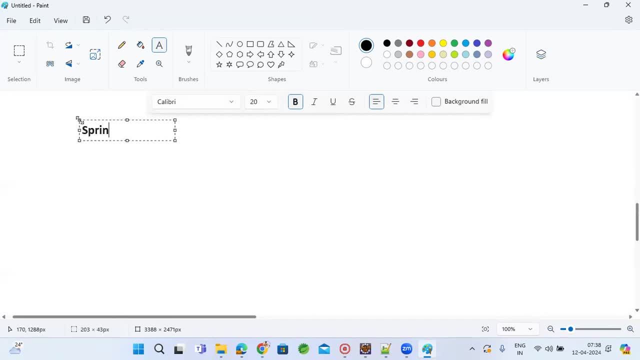 spring boot, spring boot, spring boot. they made it simple. whatever we have learned here here it will complement along with that. features. right, it is going to provide you so many defaults: starters, default configurations. basically we do lot of configurations. spring boot, you know, avoided all that stuff, so they made spring framework simple here. 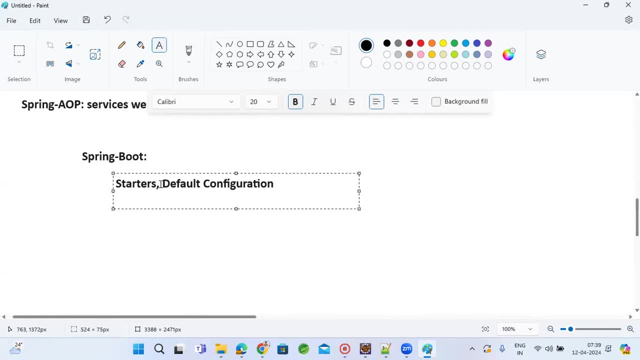 so itself. it will provide configurations itself, it will provide all the dependencies and there are some ids also to help you: scs, spring initializer and built-in embedded servers, actuators- so many such concepts we have here. you can use this as well and you can have some easy objects that we can use. 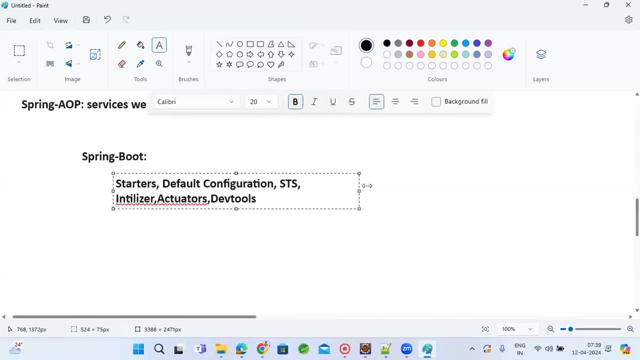 inside of it. actually, it will be a very easy one to use. let me give you a simple example of spring boot. so we have the Marchegiani array, have tools, okay, yeah, so you'll be seeing all that, how they made it simple and how to use all that features if you want to make a standalone. 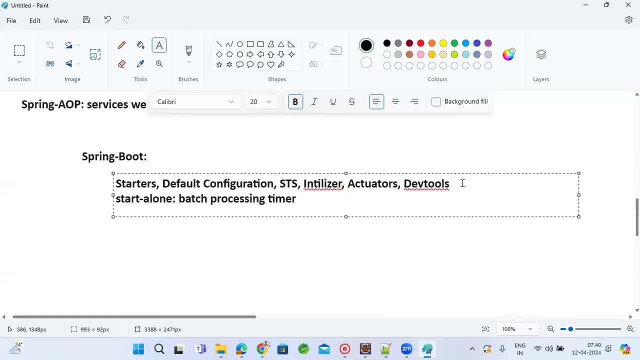 or timer applications or any standalone GUI based applications if you have, or web applications or REST applications- anything you can build in Spring Boot in you know fingertips easily. you can able to build Spring Boot based applications and lot of features we have like in Spring Boot and using Spring Boot we will learn micro services. so these two are the main two concepts that we 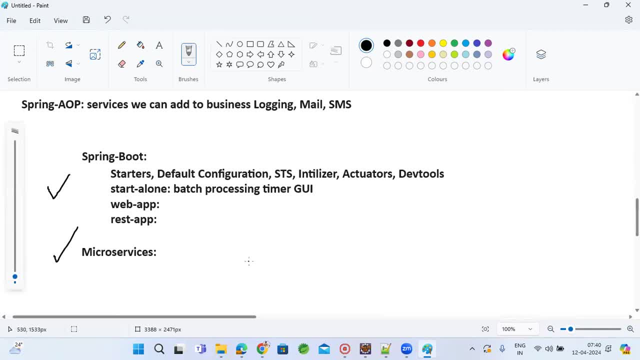 need more focus. okay, in micro services we will learn what is monolithic, what is module based application, what is service based application, how to create micro services, what are all the design patterns that we need to follow. that all will be covering in the micro services concept. spring cloud will be covered here, okay, 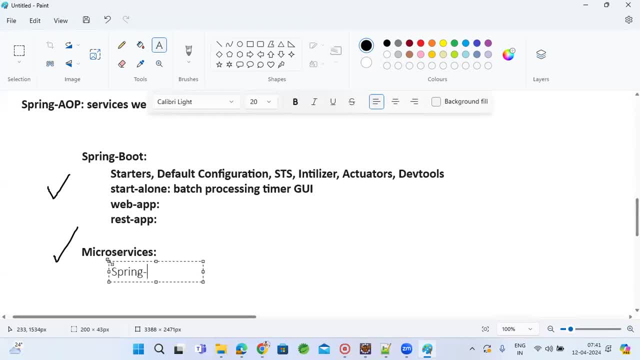 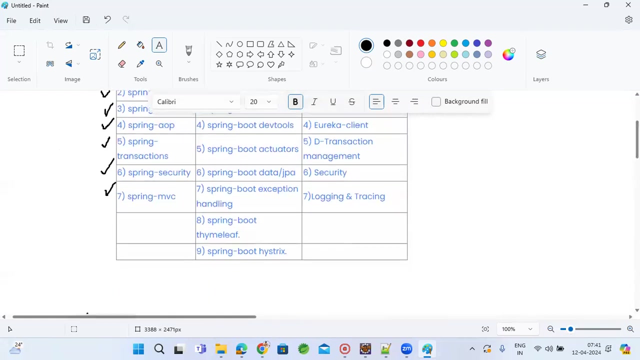 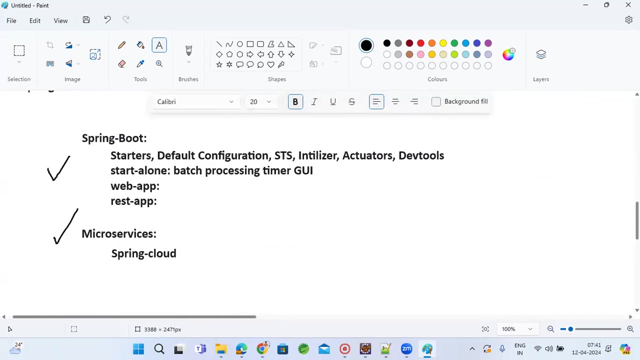 spring boot with the spring cloud concepts. spring cloud concepts will be covering it just a minute, yeah, so that is what all we are going to learn. okay, part of this session. yeah, any any questions. yeah, any any questions. uh, in that any like project will be covered. um, yeah, during the spring boot and micro service. 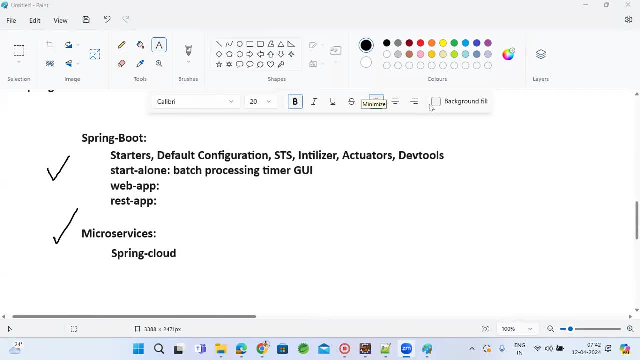 sessions. i'll be showing you small use cases, not a lengthy one, but, yeah, end-to-end use cases will be covered. okay, conclude the micro services right, especially by all the features. i'll be, uh, doing one small project, yes, okay, and completely live coding sessions only will. 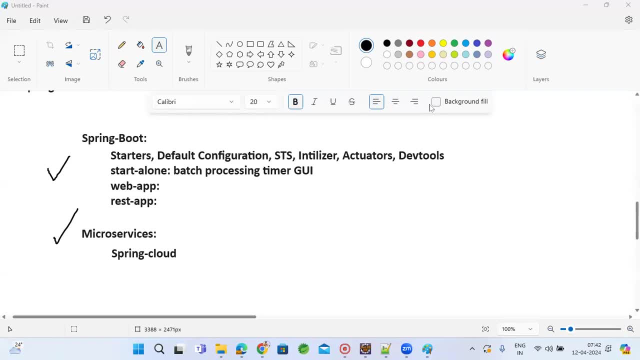 happen for every concept. right, i'll be concluding it with a code. so, end of the day, you can easily able to design a system. in case, if you want any help on the end-to-end designing system- how to write, uh, break the requirements into functional requirements and design tables and end-to-end 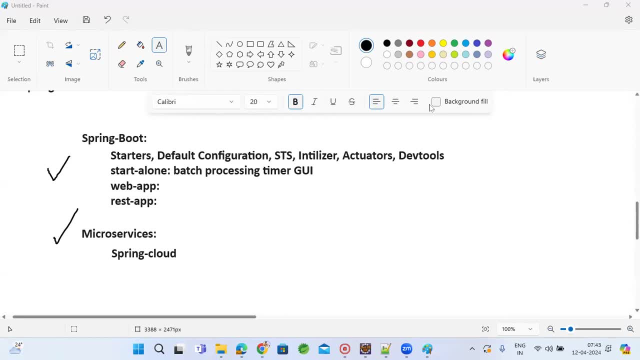 flow. i can, i can help you guys. okay, i'll take a session for that as well, okay? yeah, christopher nirmal, do you have any questions? and yeah, as i said, right, uh, uh. and classes will be daily- um, yeah, only weekdays, okay, um, and classes will be daily, um, yeah, only weekdays, okay. 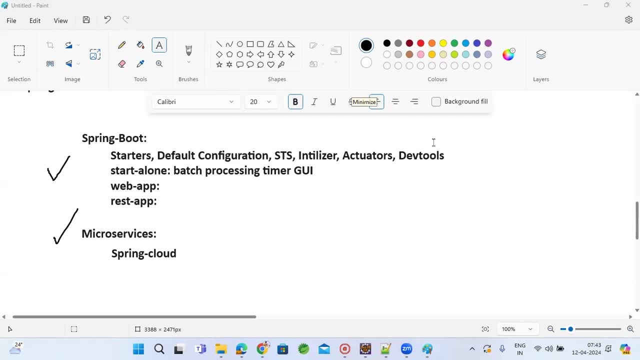 uh, weekday sessions, uh, monday to friday, and during weekends i'll be covering design patterns. apart from this, i'm going to create a solid design patterns and all gang of four object oriented patterns. object oriented design patterns also will be covered. okay, these are not part of course, but i'll be conducting free workshops and covered, okay, that will be during. 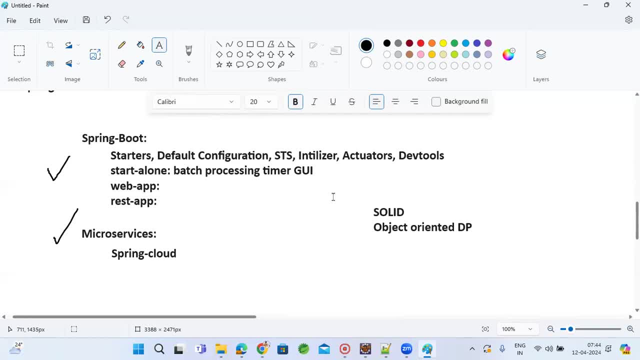 our weekends. they are very important. okay, understanding design patterns. they are very important. okay, understanding design patterns. they are very important. okay, understanding design patterns for a developer. so it will be: yeah, go ahead. so the course, the course duration. so how long will it last? two months, two months. 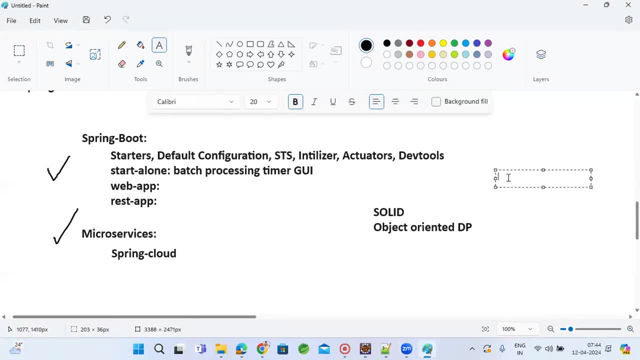 so the course, the course duration. so how long will it last? two months, two months. so the course, the course duration. so how long will it last? two months, two months, christopher almost, christopher almost, christopher, almost, okay, yeah, okay, yeah, okay, yeah. so springboard will start when like it. 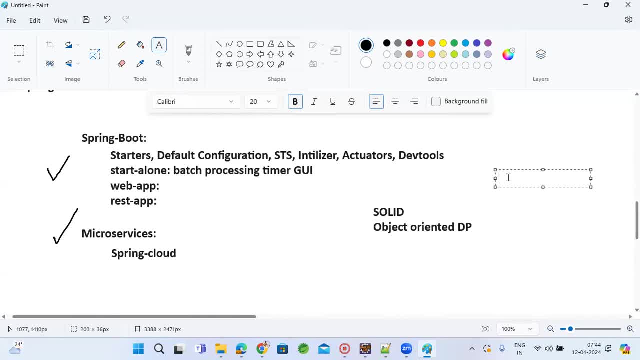 so springboard will start when like it. so springboard will start when like it will. in one month it will start or it will take time. no, it will. uh, no, spring boot will start after 15 sessions. okay, first 15 seconds i'll be covering on uh spring framework again. right, if you know spring framework, good, but still. 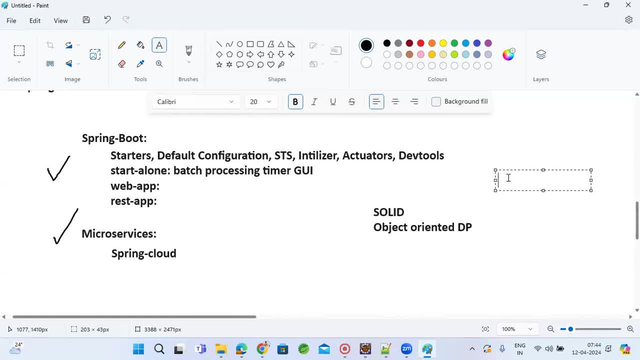 uh, my pattern is completely different. you will understand depth of spring, okay. so, yeah, uh, that's how i build a strong foundation of spring first, then we will start the spring boot. then you will feel okay, spring boot internals easily. okay, mostly i'll focus on configuration stuff. annotations in spring. 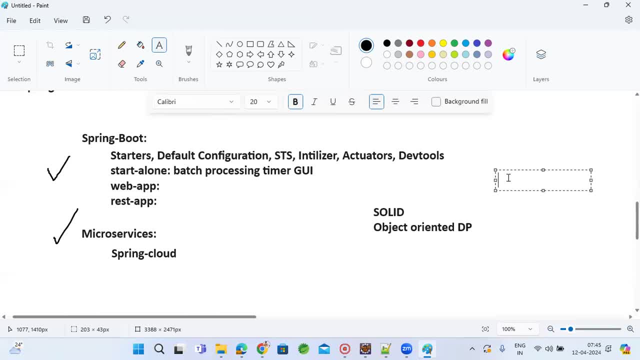 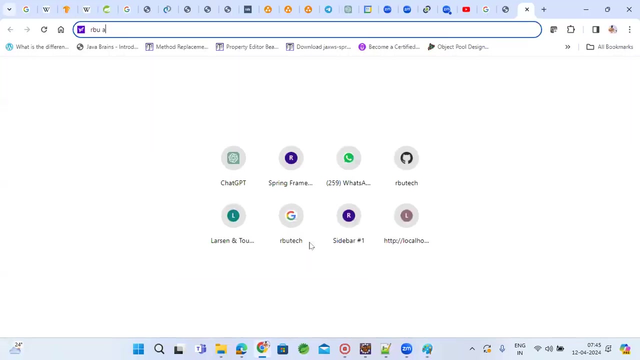 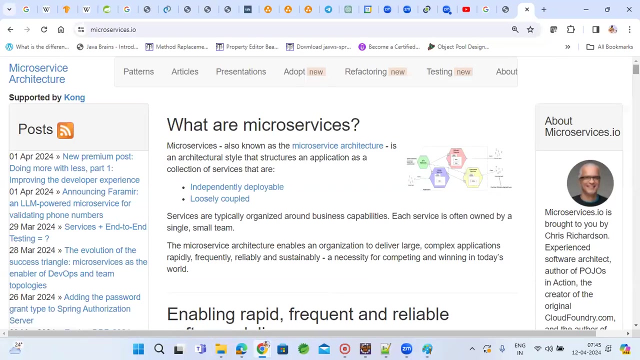 that will helps you a lot in spring boot chat. nirmal shiva, go ahead. yeah, sir, you will cover all uh design pattern. microservices, yes, uh, like circuit breaker, and eureka. eureka is not a design pattern for service discovery, we use that. okay, see, this is the architecture. i am sharing you the best design patterns. okay, uh, you can. 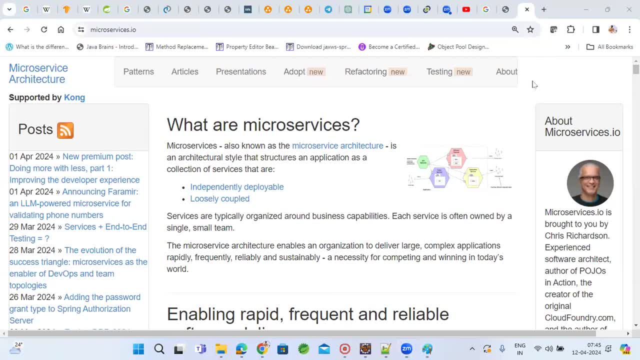 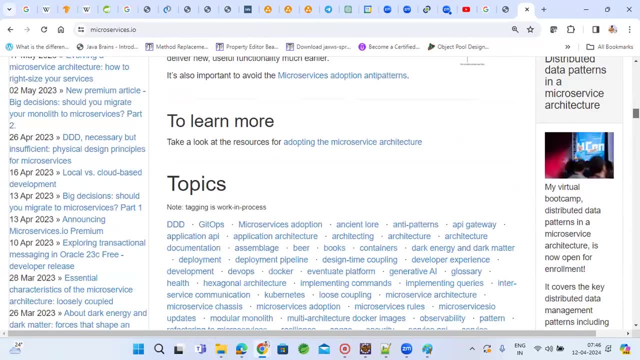 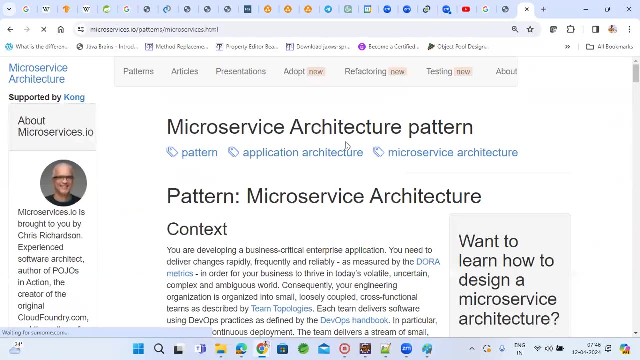 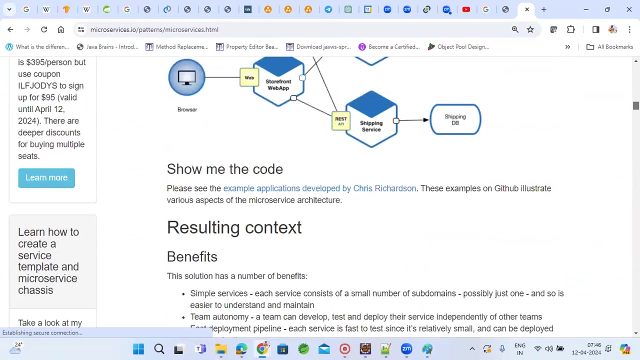 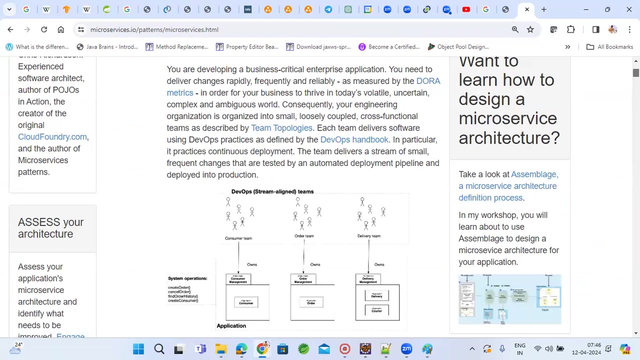 see microservices org i have shared. okay, this is the place where all experts talk about microservices. okay, here from this. okay, i'll be going to discuss all the design patterns which are required for microservices architecture from the designing first, you know, to learn design patterns- our mindset also. we need to change. uh, we should not keep our mindset like: 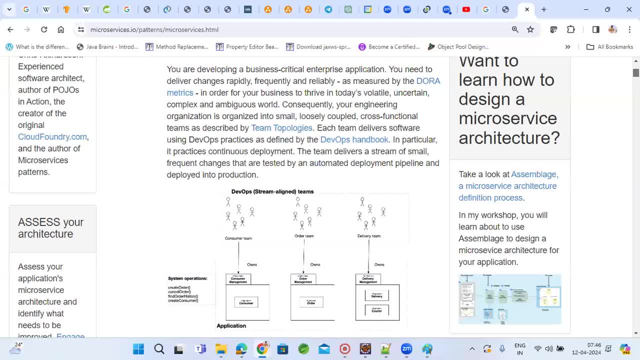 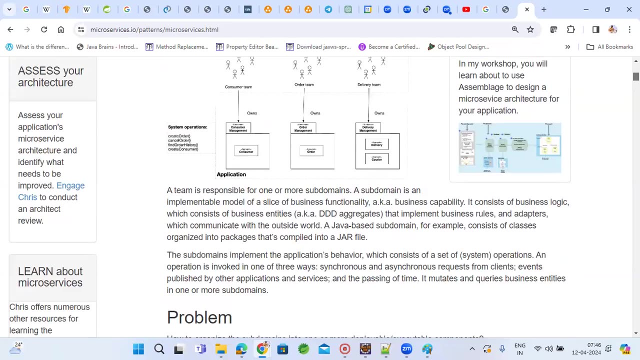 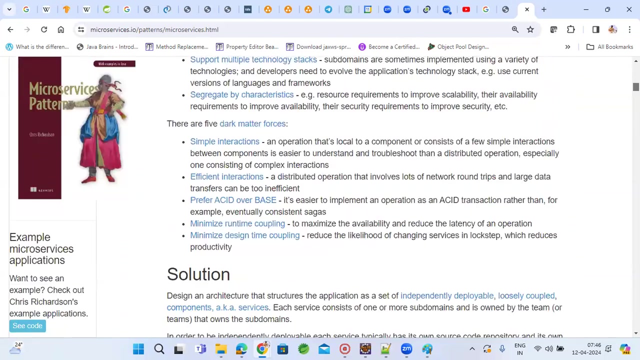 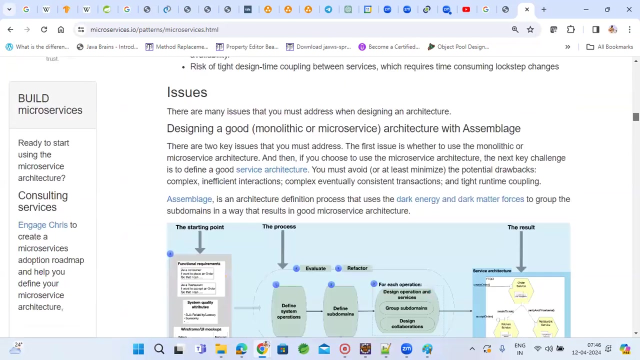 a monolithic developer. so how to you know convert from requirements onwards, how to take our requirements, uh, for micro services. how to design micro services. how to structure databases, okay. how to construct teams. also, okay. from the motivation side to complete programming side, all the patterns will be covered, okay. gateway load balancers: 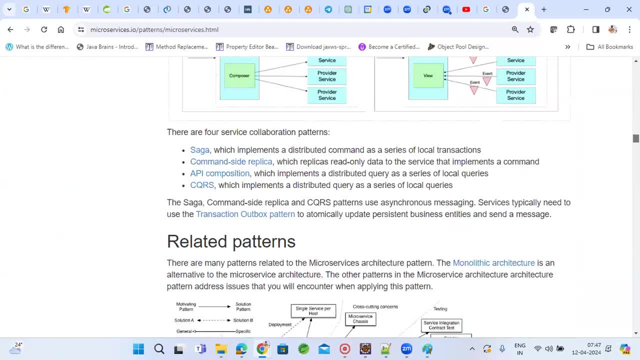 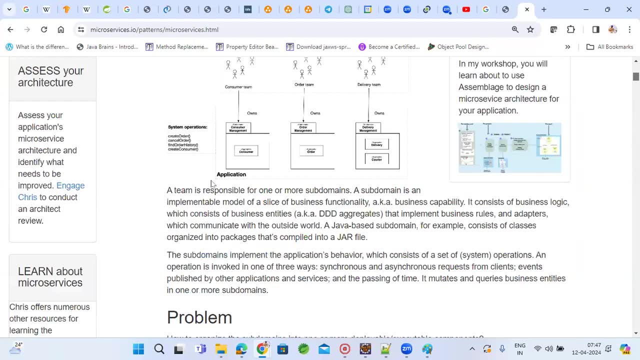 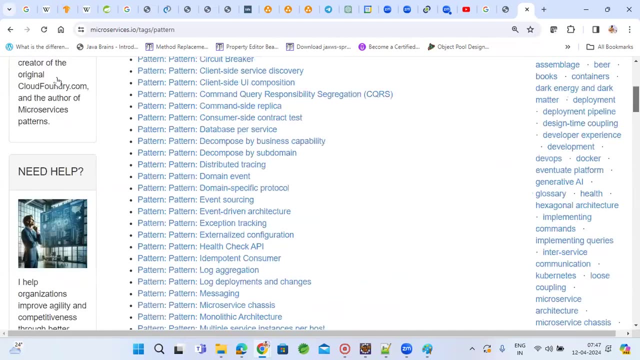 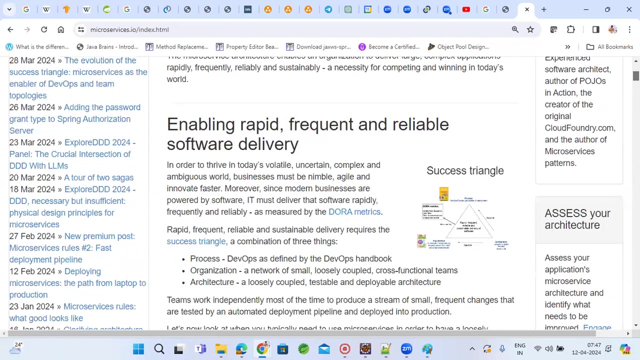 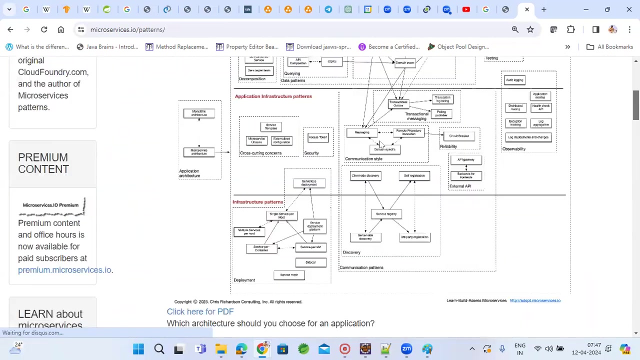 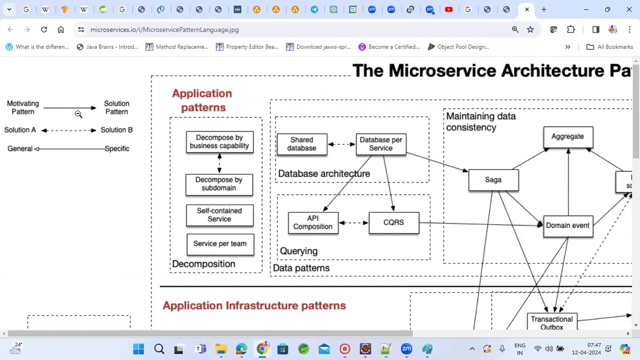 also, yeah, let me open this and logging tracing, the main architecture i want to show you. yes, here you go. yes, here you go. yeah, all the patterns, motivation pattern- see motivation patterns in in terms: right, how to understand micro services, how to convert them into solutions, okay, and application patterns. 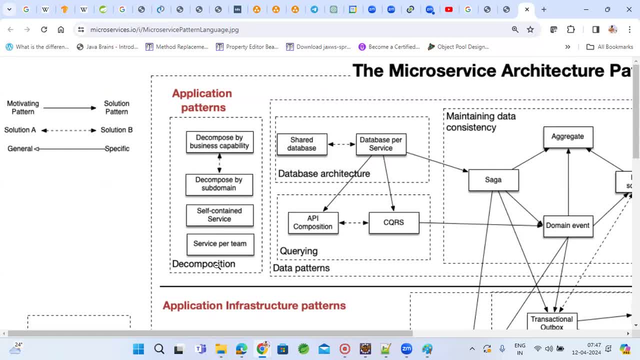 application patterns, in the sense how to decompose your requirements. i have a lot of bunch of requirements received, sir. how to now i i can decide. okay, i need to break it into this number of micro services, so which patterns i need to follow for them. decomposition by business capabilities- subdomain. 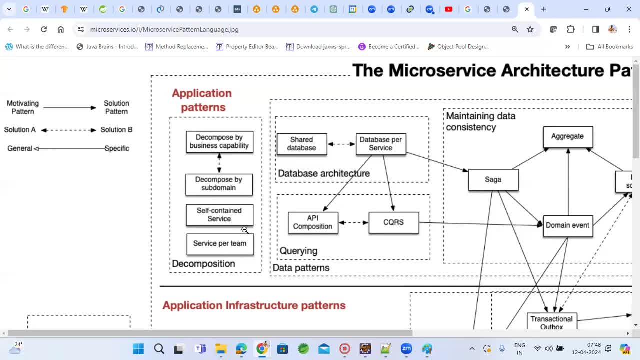 capabilities or self-contained services or services per team. okay, there are, you know, different set of rules we have. we need to know about each of them so that easily we can convert our requirement into micro service. okay, and databases. so what is the recommended shared database? do you have any idea about you meet rub s? or a database per service? and api, API composition and cqr. 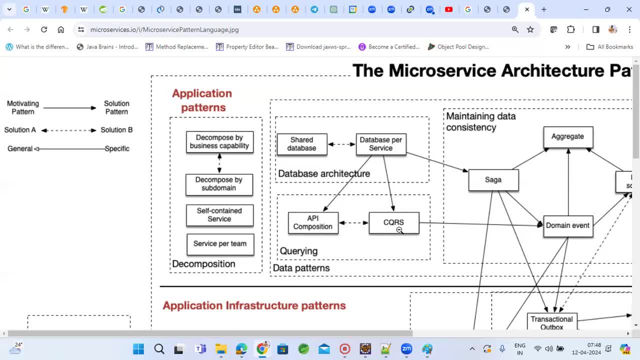 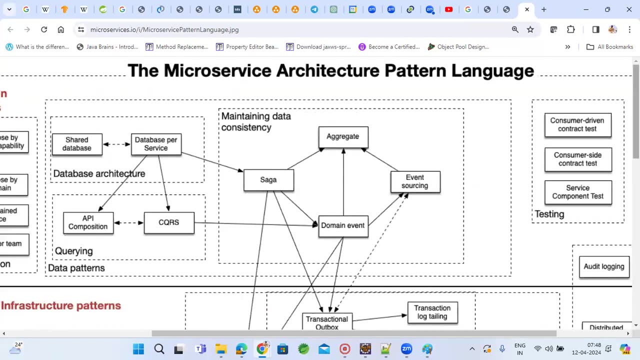 is to make you know your service database. you know save which patterns we should follow and maintaining consistency in your database- event driven or disappear which one we should follow. and testing. you know how to provide apis for testing swagger kind of contractor. eh so a couple other things, such as missions, std and 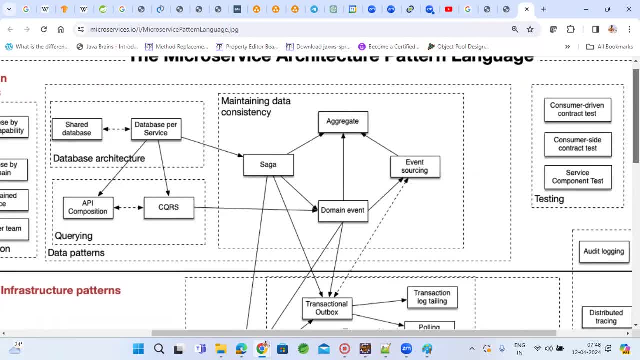 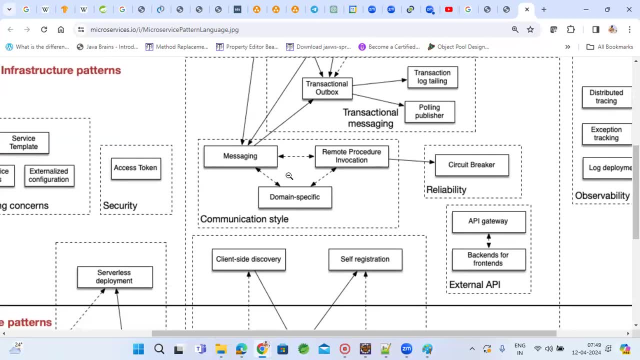 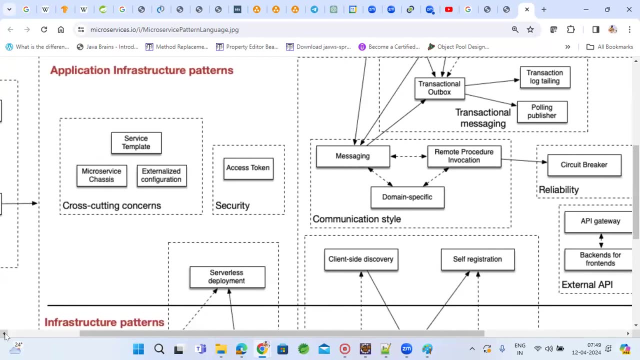 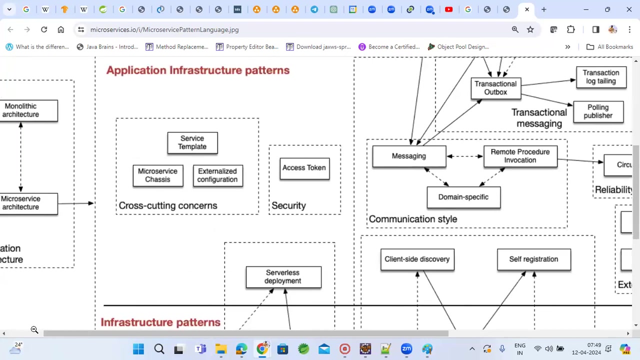 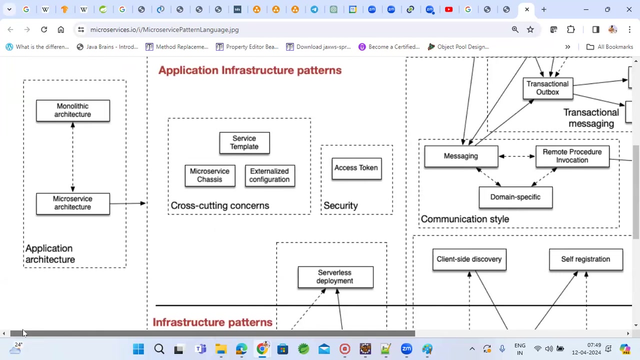 know how to provide apis for testing, swagger kind of thing will be covered. and for messaging, okay, same for event-driven architecture. how to use mq, rabbit, mq- i'll be taking there- and security in micro services, how we can adopt- uh, sir, we will cover kafka also- when we are communicate two micro services to each other. yeah, i'll use rabbit, if possible, i'll. 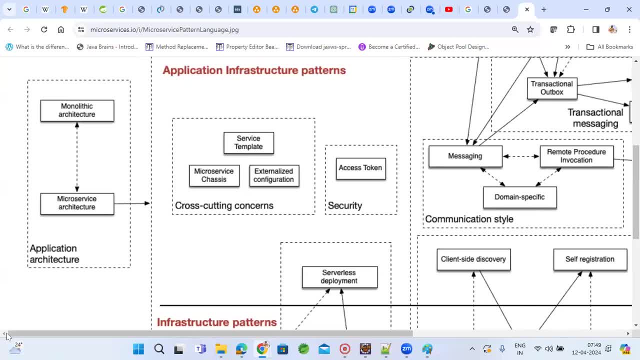 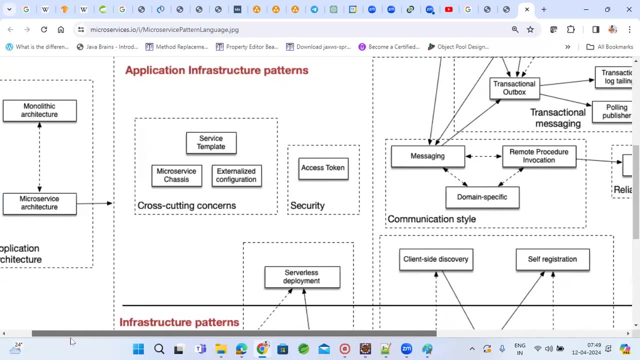 take one example on kafka also. okay, we can include, that's not a big deal. we have in spring boot itself a kafka dependency. we can add and we can check. and how to convert monolithic to micro services. there are again different design patterns for this monolithic to micro service conversion. 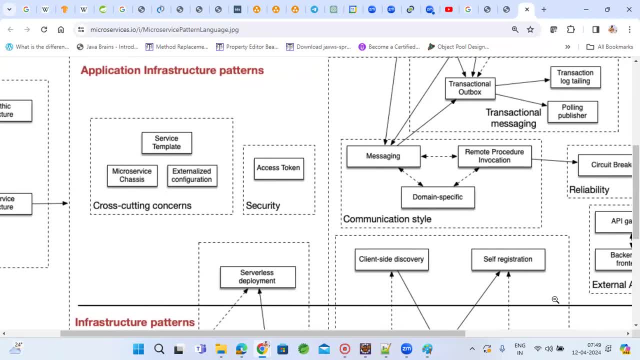 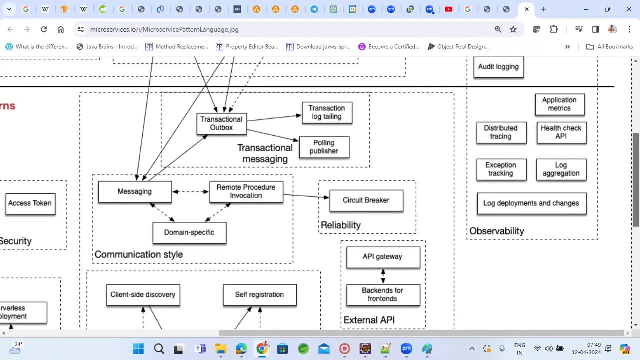 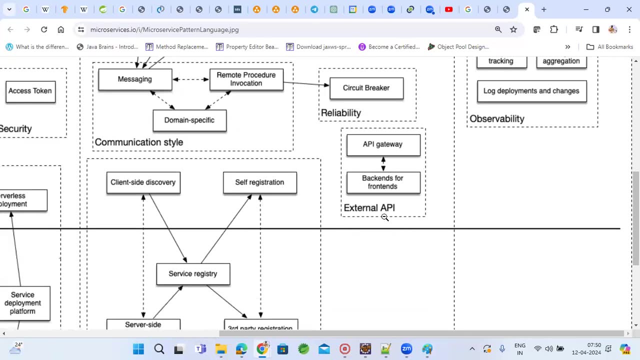 okay. reliability, okay, okay. circuit breaker: design pattern observability, logging, distributed tracing, health checks, right exception tracking. how we do all that and to give access of your micro services to external. how we use eapi gateway. and what is this pattern? backends for front end service registry and service discovery. 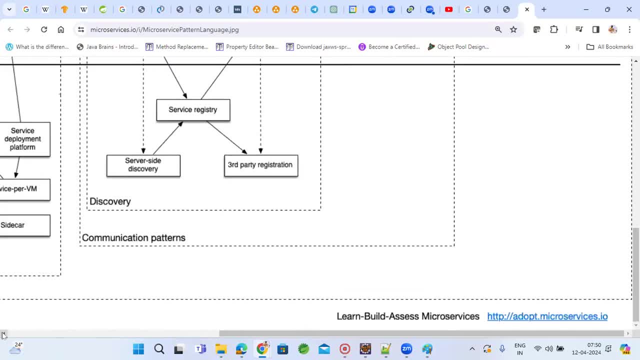 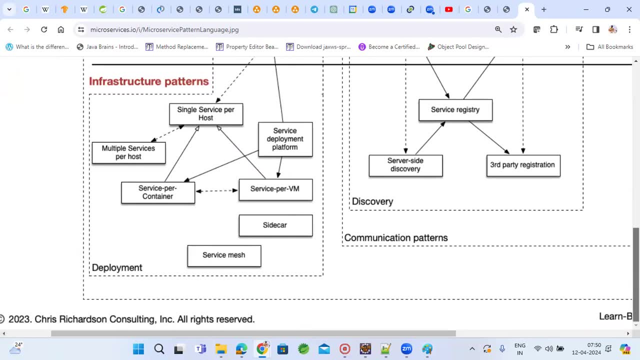 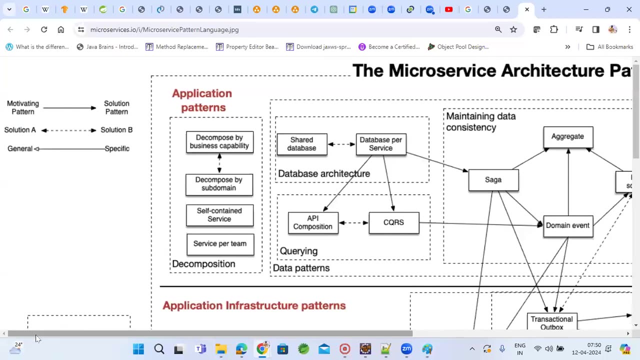 okay, how do we register our services? okay, and how we share that services with others. all these concepts, okay, all the best patterns out of micro services, right, not too complicated. i'll make them very simple and easy to understand and through examples, right, everything i'll be concluding, like cloud configurations, centralized configurations. 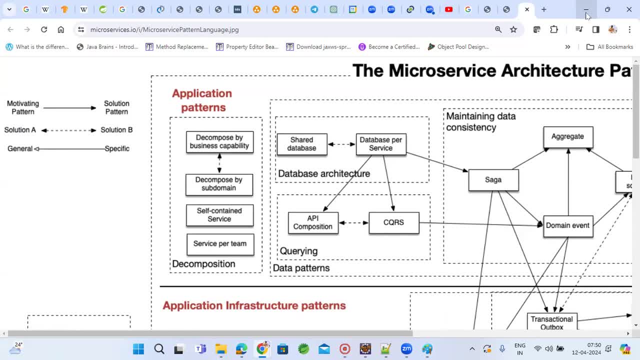 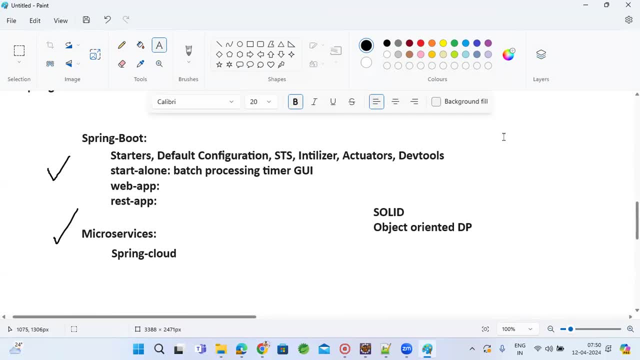 i'll be covered. so the program is simple here, okay, um, the pattern also simple. just if you can spend these 45 sessions, you can easily understand. so daili. uh, this recording also right. videos will be shared with you. okay, video recordings will be available to you post to session. 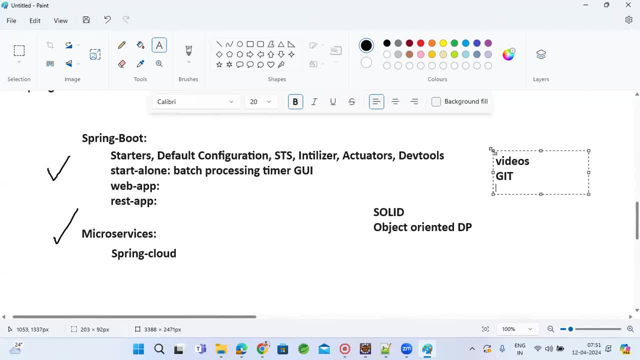 and the examples i'll upload into git so that examples also you'll get, and my ebook also. i'll share it with you, okay, and if you struck anywhere, you can reach out to me anytime. i'll be available right at this moment you get statistics and you get information that you get information from the site that you can通 поговор know what is this we're talking aboutINFOз. 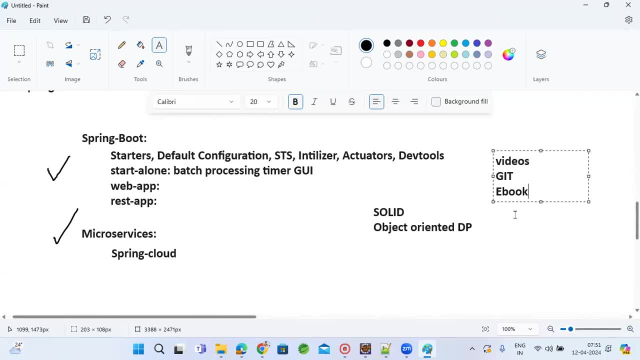 so i want to thank our partners and you want to praise them to help us. Southern Lakshmet recommend it by email. we do, but i want to acknowledge that you are here. reach out to me anytime, i'll be available, okay. so that is the pattern, guys. 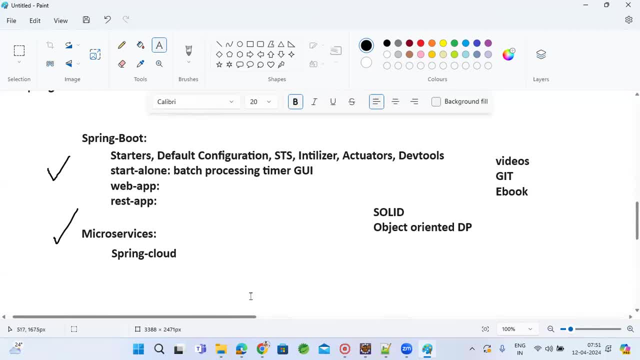 and the session will be one hour only daily. one hour to one and a half hour, depending on the session. in that one hour itself, we are going to jumping into a lot of coding. okay, so i'll be concluding each topic with the, you know, coding examples. okay, okay, so i can. i can only attend for one hour. 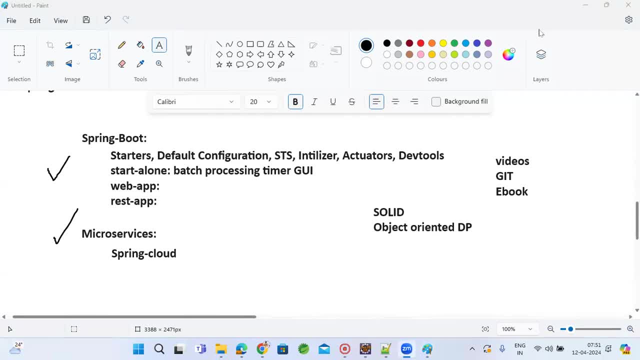 yeah, yeah, mostly it will be one hour only. okay, yeah, as and when required i may extend, but yeah, mostly one hour, because i'll have a next session. post your discussions, okay, yeah, what i would recommend you is just ping me on this number. i'll create a group and 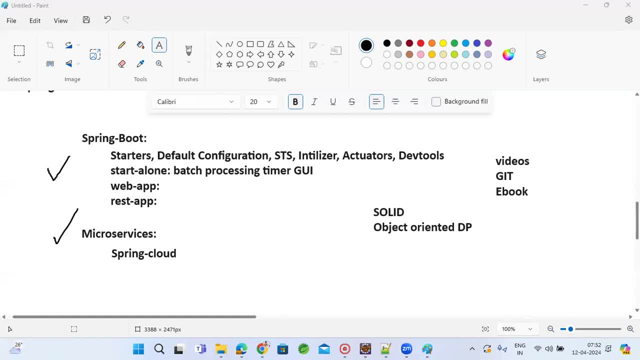 add you to the group and i'll add you to the group and i'll add you to the group. you there, i am pinging my number. okay, immediately text me. nine one, eight, two, double six, two four eight two. yeah, i shared my number, just ping me. uh, say hi, i will add your number to a group, okay. 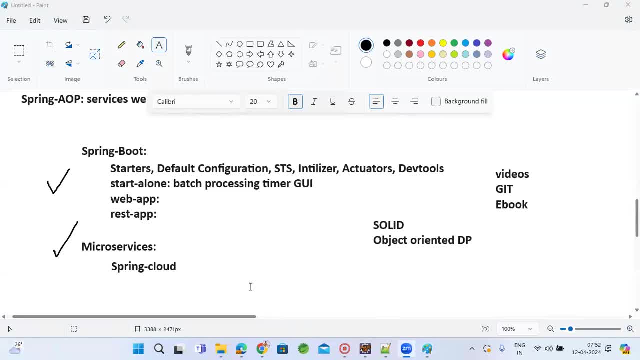 are we going to cover some testing, exactly marketo we'll be seeing here, okay, uh, yeah, i'll cover a small project with the tools. okay, i'll cover a small project, a simple project i'll take with the tools, uh, the mandator tools like sonar, how to use sonar, cube, marketo based testing. 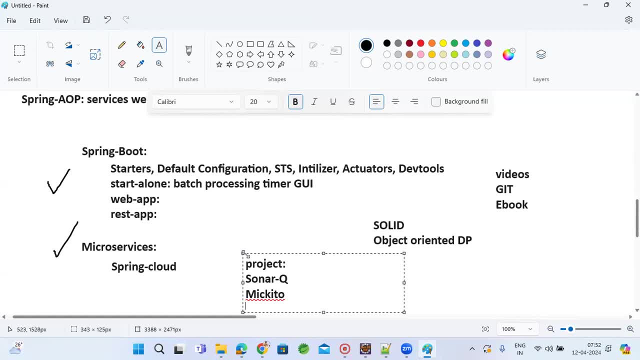 okay, uh, the basics. okay, how to, uh, you know, use git, git pools and compades, jenkins. i can't do setup, but i'll. i'll give you, uh, how jenkins work. okay, how to pass. you know runtime parameters there. okay. uh, how devapps cacd will work. i'll explain.